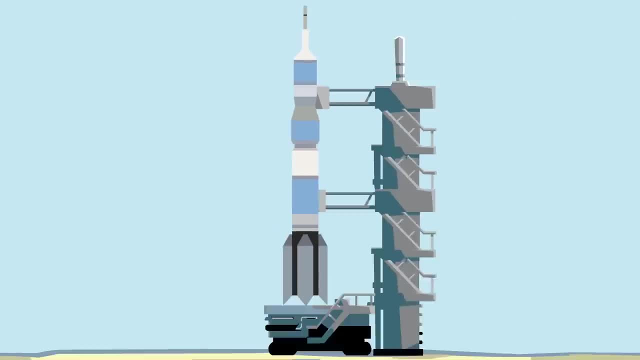 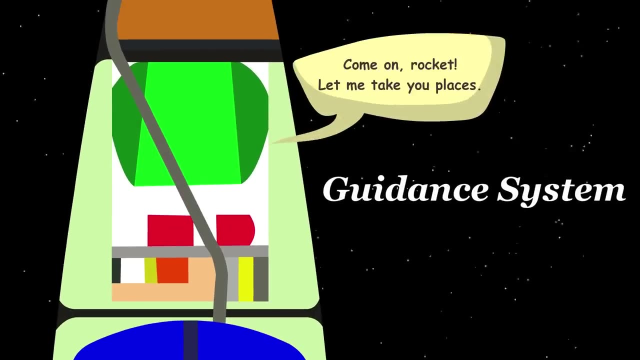 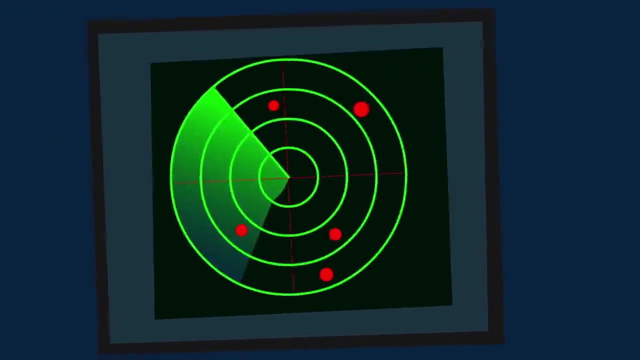 then the payload would consist of a missile. Next is the guidance system, the system which ensures that the rocket stays on its intended trajectory and goes where it's supposed to go. The guidance system consists of onboard computers and sophisticated sensors, as well as radar and communication systems to maneuver the rocket while in flight. 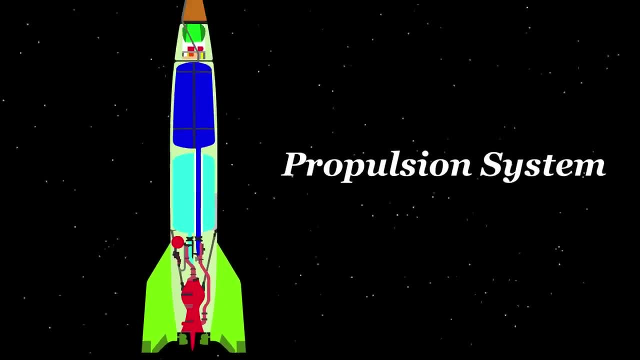 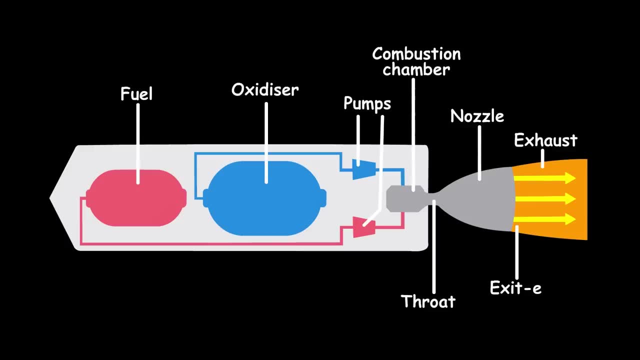 Last is the propulsion system. A majority of the entire length of a modern rocket is actually made up of the propulsion system. As the name suggests, the propulsion system consists of the components that help launch the rocket off the ground and subsequently propel the rocket in a given direction. 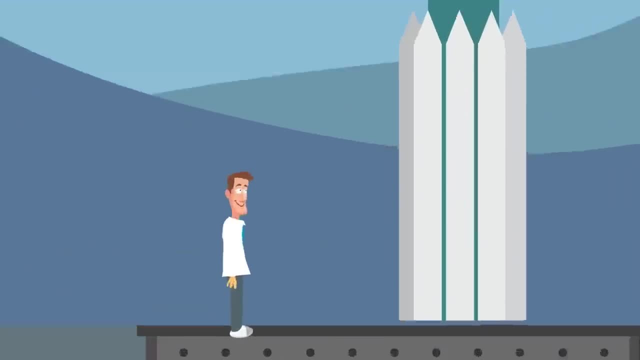 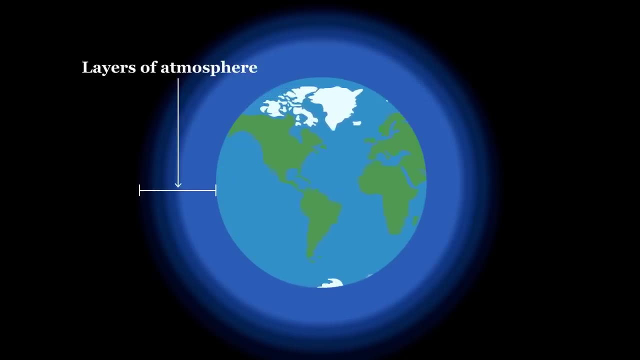 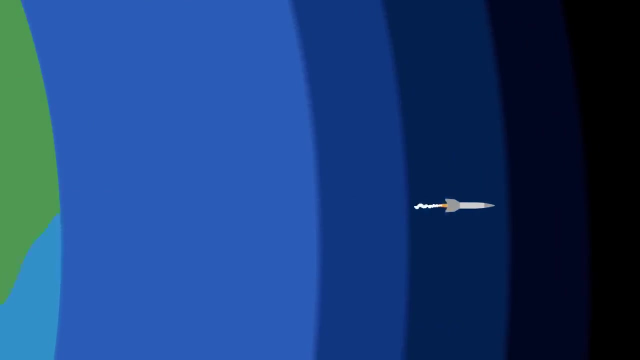 So how is this huge, enormously heavy cylindrical metallic tube shot into space? In order to get into space, the rocket must first cross the thick layers of atmosphere that envelop our planet. Since the atmosphere is thickest near the ground, the rocket has to go extremely fast in order to get past this part of the atmosphere. 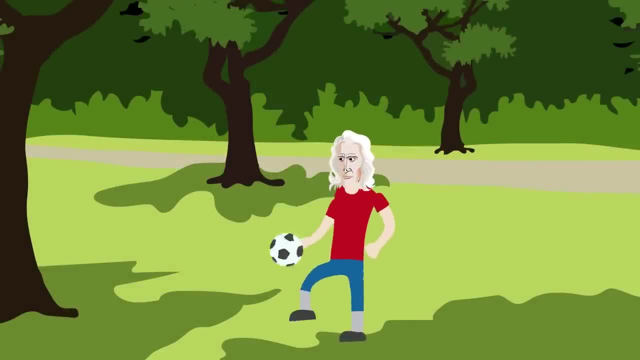 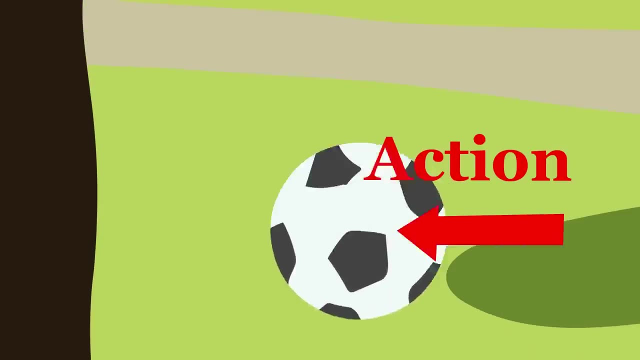 So how does it climb so fast in the air? The answer to this question lies in one of the most popular physical laws of the universe: Newton's third law of motion. According to the third law, every action has an equal and opposite reaction. 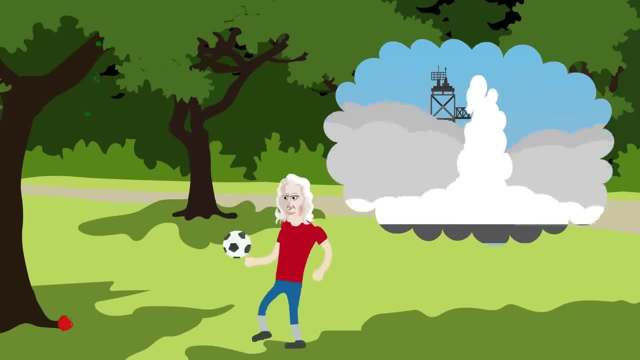 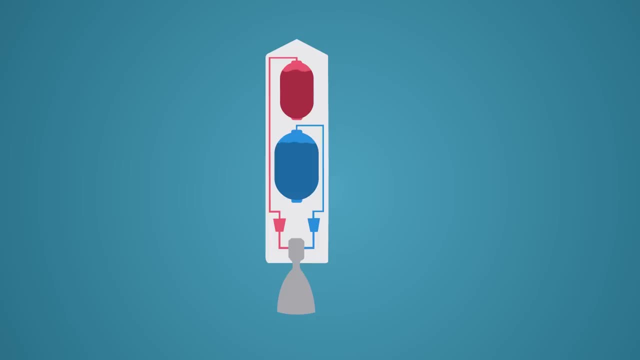 In our case, we have a rocket that we want to launch into space. How does the third law help us? That's where the rocket engine comes into play. A rocket engine works by burning either a liquid or solid fuel in the presence of an oxidizer. 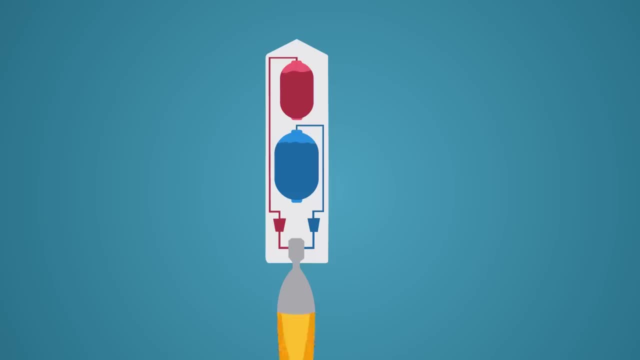 When the combustion reaction occurs, it throws out a great deal of mass as a byproduct of the reaction. These byproducts are released at great speed through the bell-shaped nozzles that you see at the bottom of rockets, Since the rocket pushes the exhaust down. 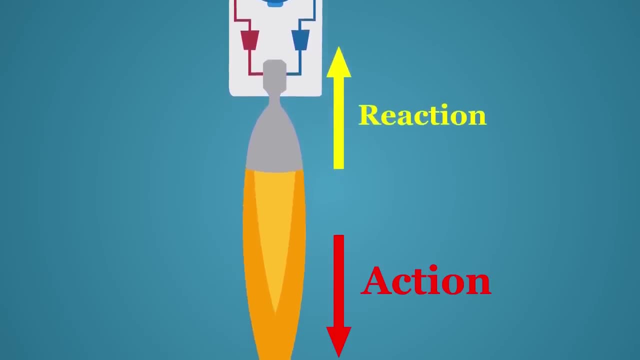 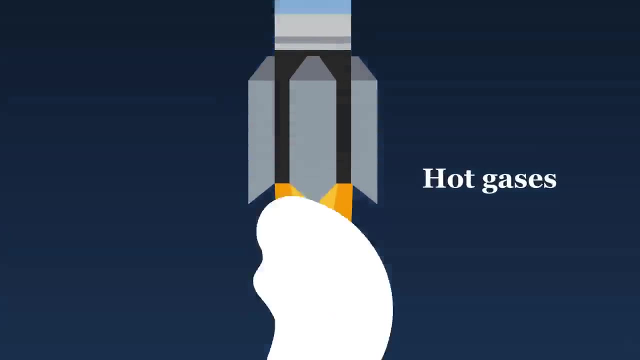 the exhaust responds by pushing the rocket up at great speeds, which lifts the rocket off the launching pad and propels it upwards into space. In a way, you could say that a rocket shoots upward by throwing hot gases from its exhaust nozzles below. 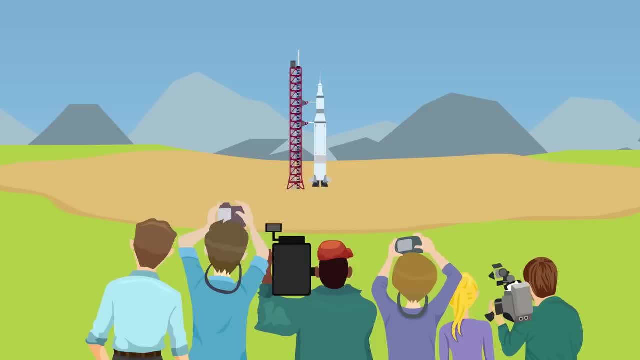 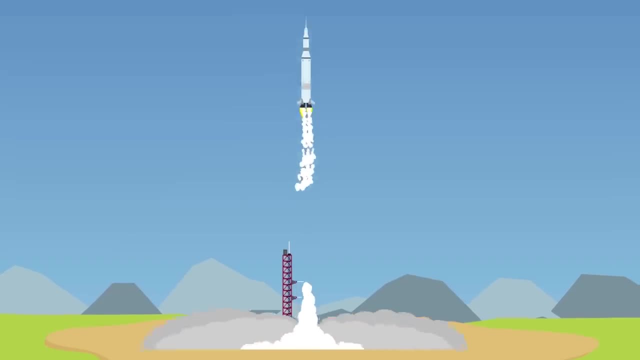 If you have ever seen a rocket launch in person, or even seen a rocket launch video on the internet beyond the lift-off phase, you may have noticed that a rocket doesn't maintain a straight trajectory all the way up. It lifts off perfectly vertically.